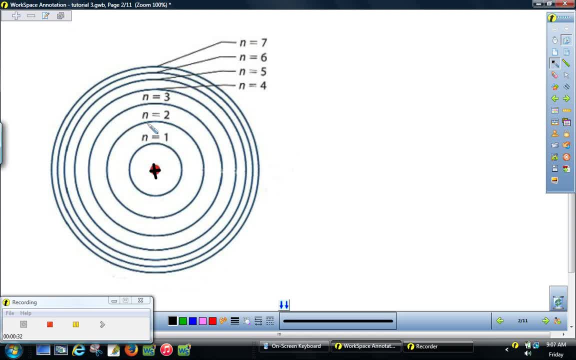 And we had a positive nucleus in the center and then he thought that the electrons were traveling around the nucleus in these fixed orbits. He was incorrect in that they're not traveling around in fixed orbits, but he was correct in that there are different energy values for the electrons. 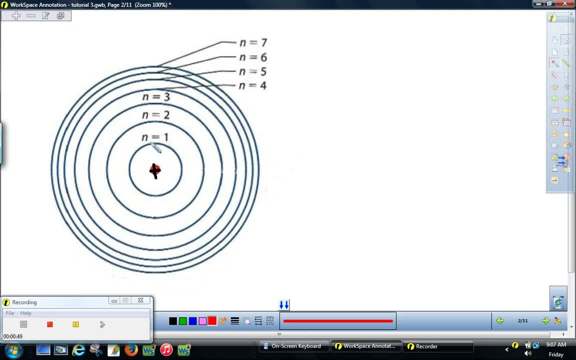 So electrons found in the first energy level- the first ring- are going to have a certain amount of energy, And then electrons found in the second energy level are going to be farther away from the nucleus, And the reason why they're farther from the nucleus is because they have more energy. 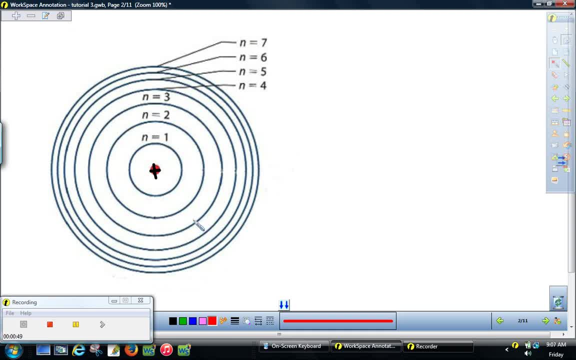 So there's a value associated with electrons and how much energy they have in the second energy level And then in the third energy level they have even more energy than the second and first, And then, as the electron continues to move outwards and is found farther away from the nucleus, they have to have more and more energy. 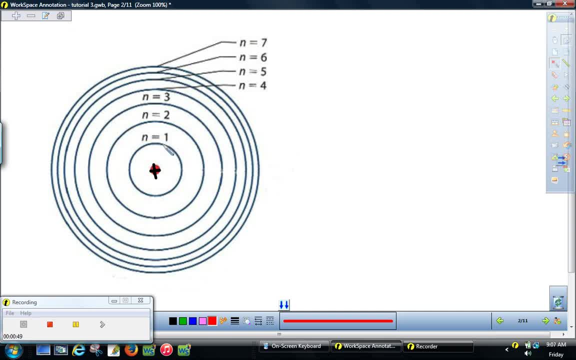 And so electrons in the seventh energy level will have more energy than the electrons in the first energy level, because they're trying to resist the protons. The protons are trying to pull the electrons into the nucleus, And so the more energy an electron has, the more it can resist. 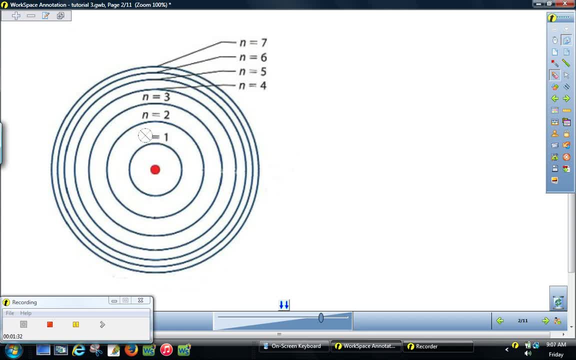 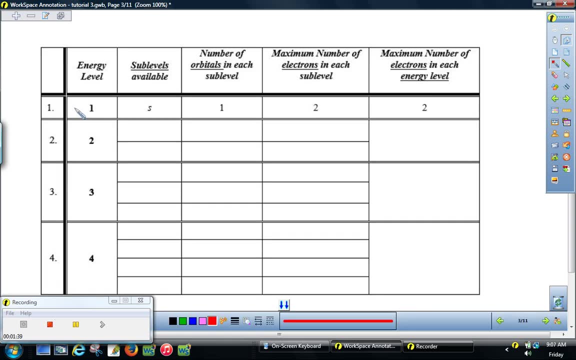 And the farther it can be found away from the nucleus. All right, so we have seven energy levels, or seven different distances away from the nucleus. That's the first step. So when you see energy level on this chart that we're going to fill in together: energy level one, two, three, four- this is closest to the nucleus. 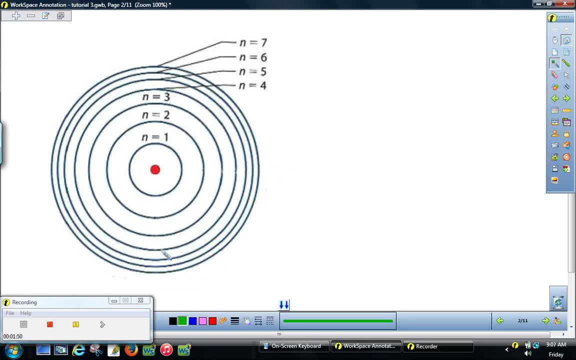 And then something else I want to mention too is the first energy level. look how tiny it is in comparison to the other ring. So there's not much room for the electrons, whereas the second energy level- it, has much, much more room. 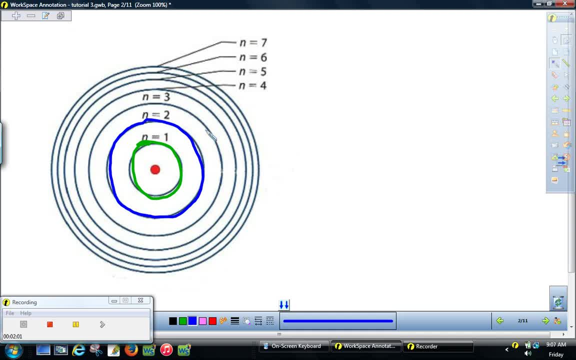 And so this is two-dimensional, but remember, atoms are actually three-dimensional. So there's a tremendously amount more room for electrons to move around in the second energy level than the first, And that's why more electrons can be found in the second energy level. 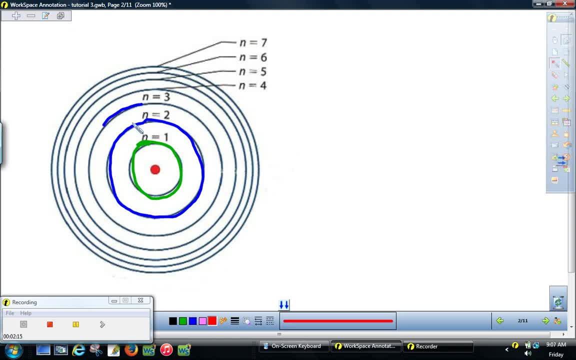 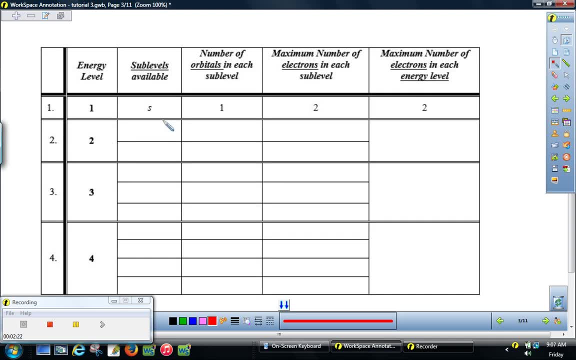 Third energy level is even bigger than the second, So even more electrons can be found here in the third energy level or farther away from the nucleus. So let's look at this chart. So the first energy level has S sublevels and S sublevels only. 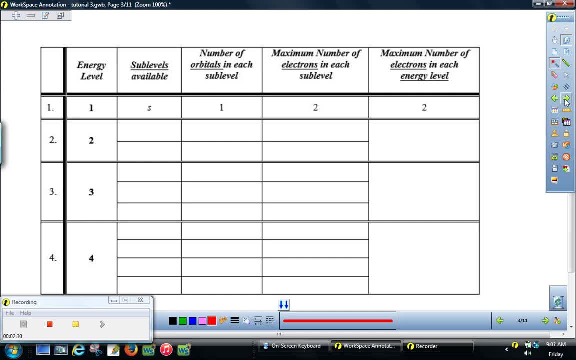 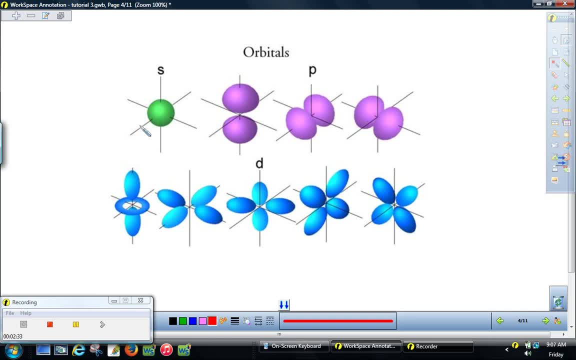 And so this S gives us an idea. This is the shape of the region that the electrons are going to be found, And so this diagram shows us that the S is spherical, looks like a circle, looks like a ball, And so we have the X, Y and Z axes. 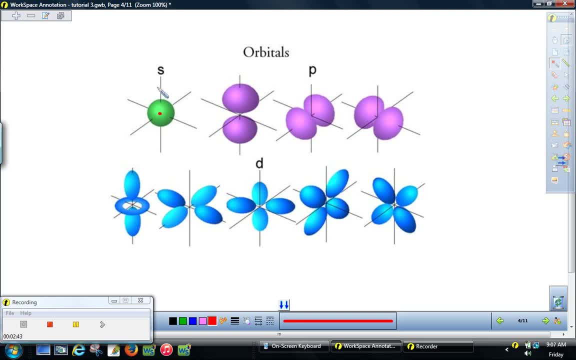 Where these three axes intersect, right here where my red dot is, that's where our very tiny, dense, positively charged nucleus is. So this green shaded area tells you the approximate region in which electrons will be found, if they're found in the S sublevel. 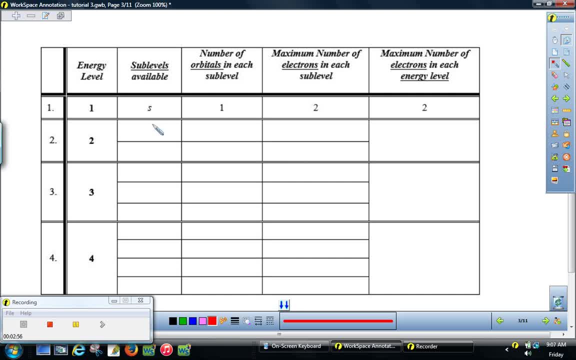 All right. So each sublevel can hold a distance, Different amount of electrons. The S only has one shape or one type of orbital, And we'll talk more about that. So each orbital can only hold two electrons. So every orbital can hold two electrons. 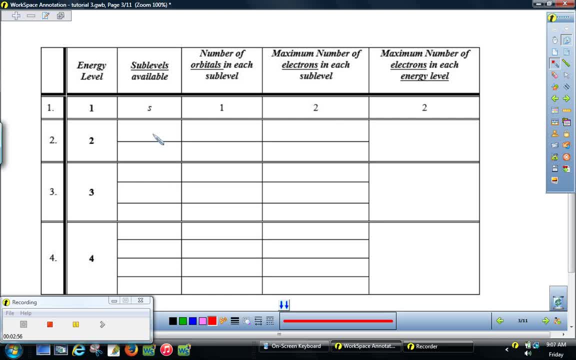 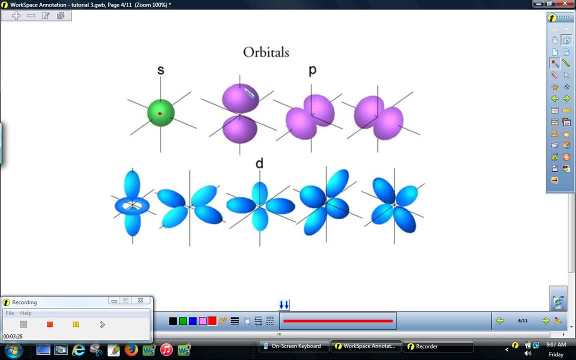 So the first energy level can only hold two electrons. Second energy level has both S spherical shatomes And there's only one type, one orbital, And that orbital can hold two electrons. But the second energy level is bigger, And so the second energy level has one. 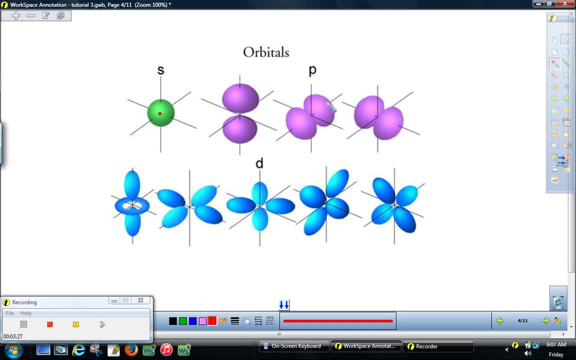 And so the second energy level has one, And so the second energy level has one, two, three orbitals. Each one of these models represents an orbital, And so what's different about these three? Well, the P. the P looks like a dumbbell. 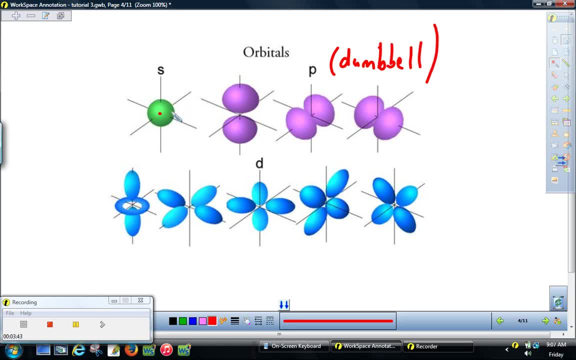 So the dumbbell shaped orbital is, you know, different than the spherical shaped orbital, So it refers to different pockets of space around the nucleus. Once again, the nucleus is right here where all the axes intersect, And so the 2P. there's space above and below it. 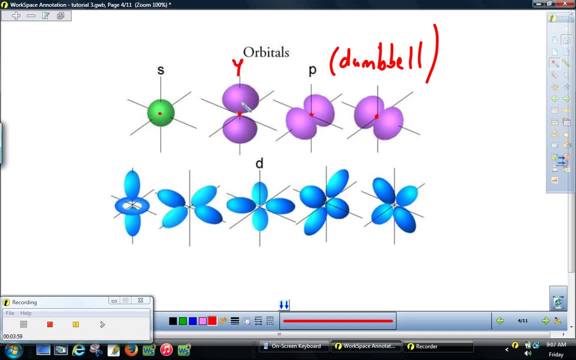 So this is the Y axis. So this is the 2P, The Y axis. It falls on the Y axis. One electron can go here. One electron can go here, So we have room for two electrons. This is the third dimension, the Z axis. 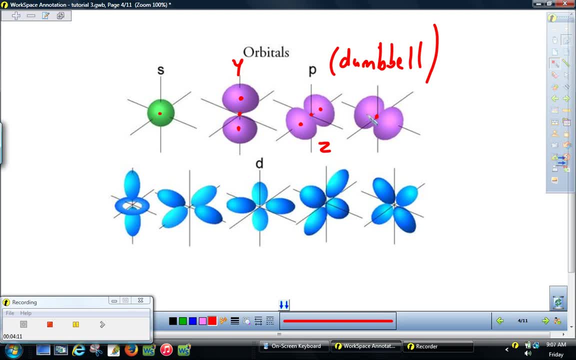 And so an electron can go here. An electron can go here in front and behind the nucleus, And an electron- this is the X axis. An electron can go here to the left and to the right of the nucleus. So we have three dimensions. 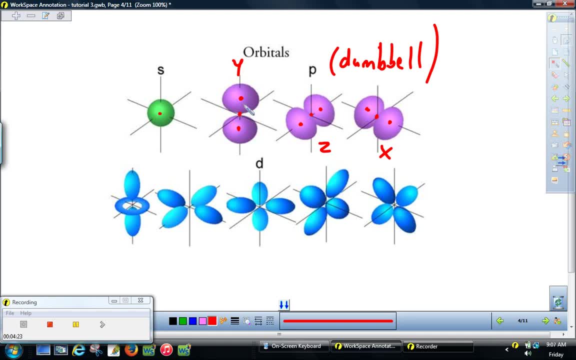 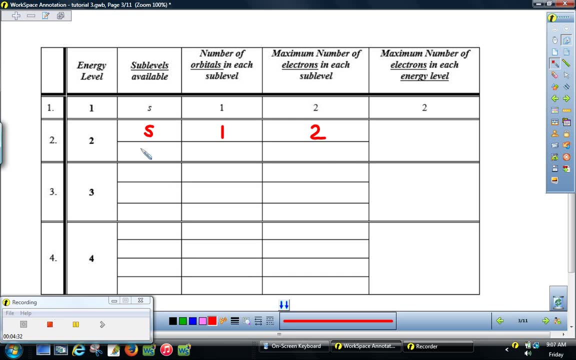 Each orbital falls on one of those axes, And so Y axis, Z axis, X axis, Each one can hold two electrons. So 2 plus 2 plus 2 is 6.. So if you come back here, P sublevel shaped like dumbbells. 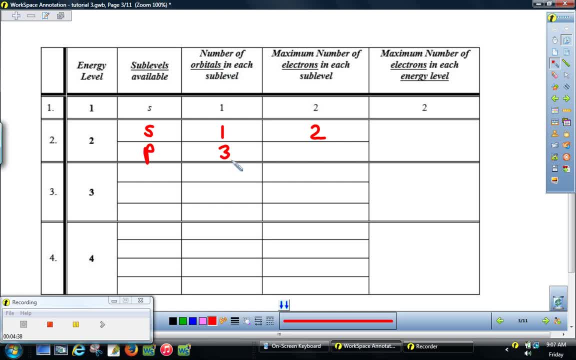 Three orbitals: the one that falls on the X, the one that falls on the Z, the one that falls on the Y axis. Each one can hold two electrons, for a grand total of six electrons. 2 plus 6 gives us a maximum number of eight electrons in the second energy level. 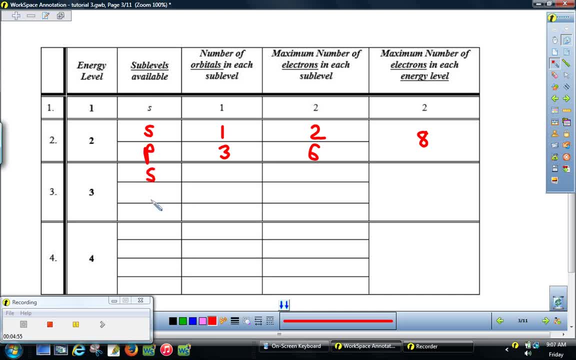 The third energy level is even bigger. So, just like the second energy level, there's going to be S And there's going to be 2. And there's going to be 3. And there's going to be 4. And there's going to be 5.. 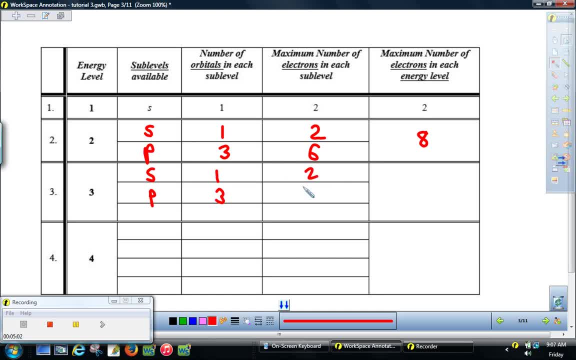 And there's going to be 6. And there's going to be 7.. There's going to be 8. And there's going to be 9.. There's going to be 10.. There's going to be 11.. 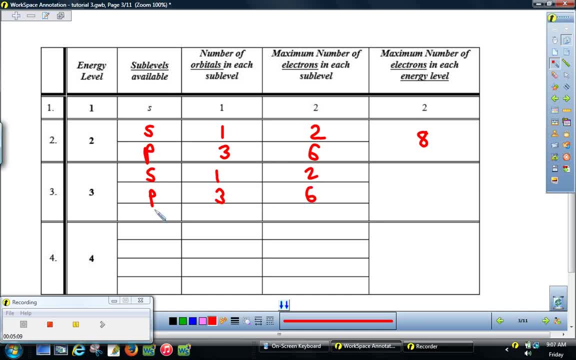 There's going to be 12.. There's going to be 13.. There's going to be 14. And there's going to be 15.. There's going to be 15.. So there's three types of P's: X, Y and Z. 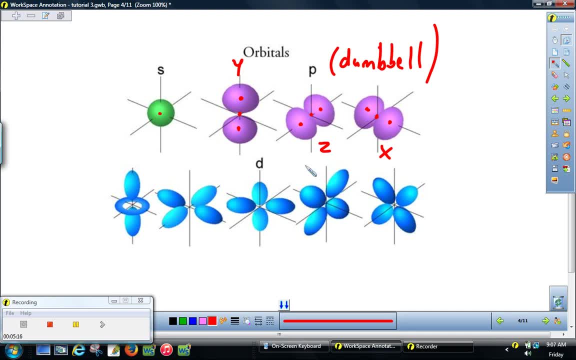 Each one can hold two, So the numbers stay the same. However, we have room for a third type of sublevel, So there's additional pockets of space that can hold electrons, And we call these the d-orbitals, So even more complicated. 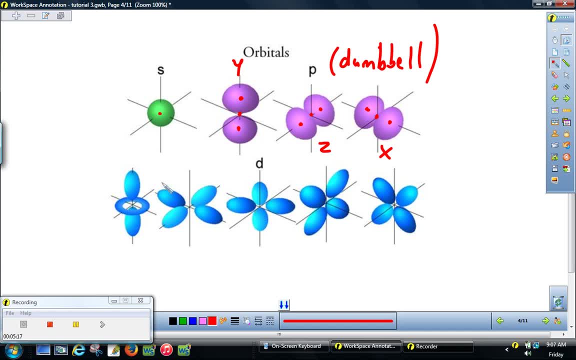 So these are like double dumbbells, or we call them fan blades, And so each one represents one orbital, one different region of space within the atom that can hold electrons. So two electrons can go in this space, two electrons can go in these shaded regions. 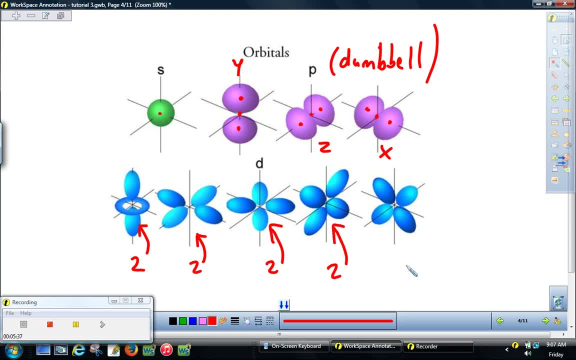 two more electrons can go in these shaded regions, two more electrons can go here in these shaded regions, and two more can go here. So five orbitals, five different regions that make up the D sublevel. Each one can hold two, so five times two is ten. 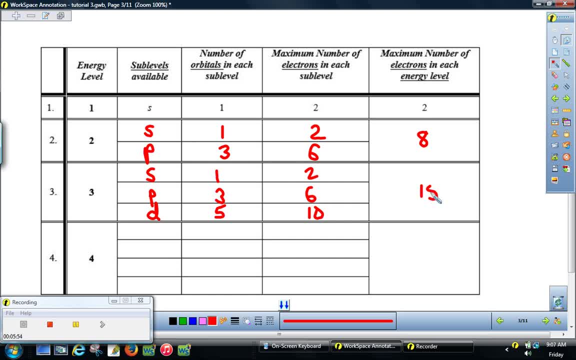 So two, six, ten grand total eighteen. So up to eighteen electrons can go in the third energy level in the third ring And then the fourth energy level and the fifth, the sixth and the seventh all have four types of sublevels. 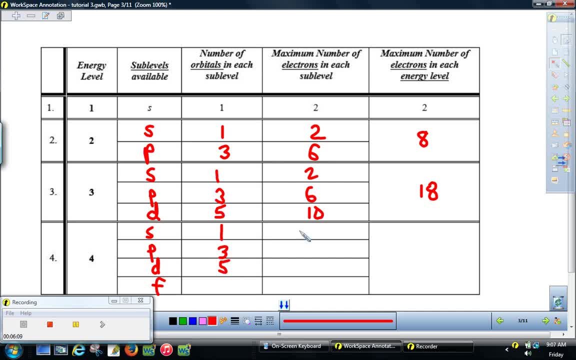 Just like before, S's have one orbital, P's have three, D's have five. Each orbital can hold two electrons, And so we get two, six, ten for the amount of electrons. The F is even more complicated. It has seven different orbitals. 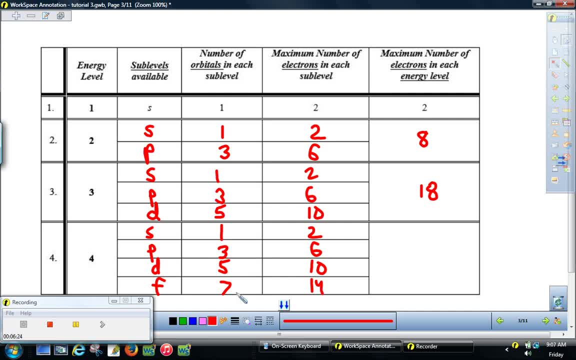 Each orbital can hold two, So a grand total of fourteen electrons can go in the F, And so if we add it together, two, six, ten, fourteen adds up to thirty-two. So energy level four, five, six, seven can hold up to thirty-two electrons. 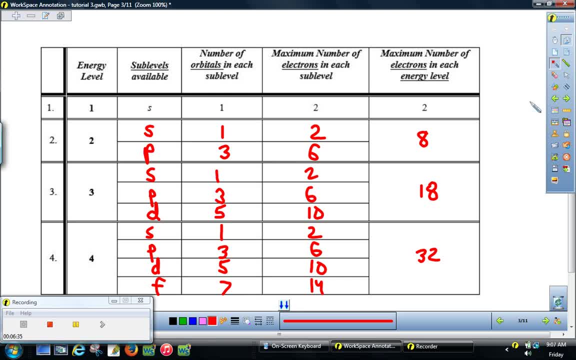 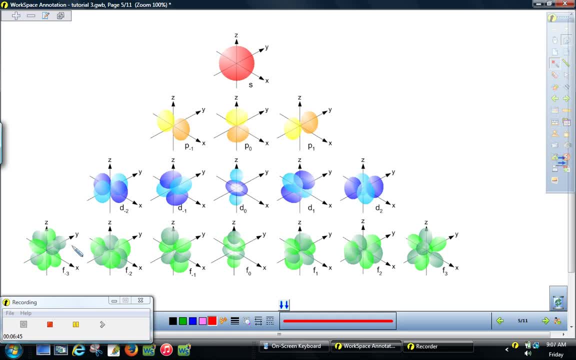 In theory, energy levels five, six, seven can hold even more, but we don't have any atoms that add more than thirty-two. So what does the F look like? Pretty tiny here, but this is one orbital. two electrons can go here.